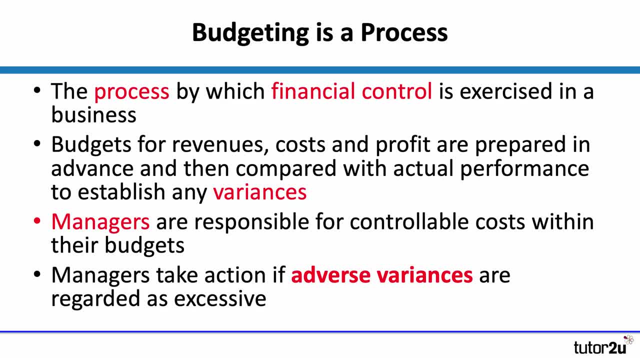 business, not just the finances. I've mentioned that budgeting is a process- Typically it's done each year and it's a way in which financial control can be exercised by the management of a business, And therefore it's a very important part of management control. What we do is we. 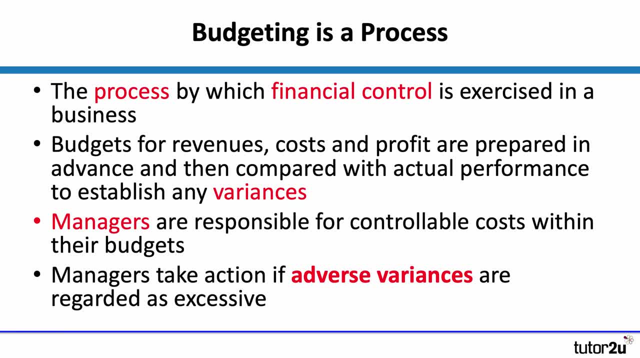 establish budgets for revenues and for the costs of achieving those revenues And therefore, if we've got a budget, we can budget for the costs of achieving those revenues. And therefore, if we've got a budget, we can budget for the costs of achieving those revenues. And therefore, 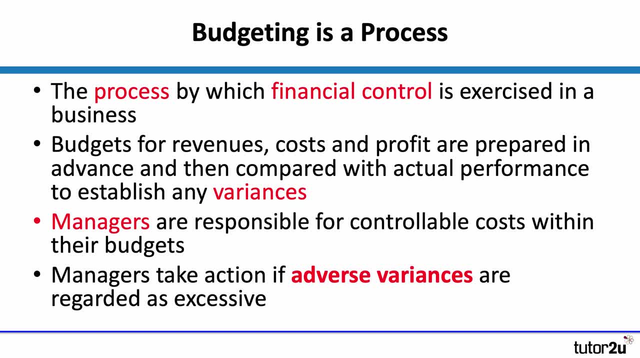 what revenues and costs, what the profit of the business is going to be. And then, as we go through the year, we compare actual performance with the budget to establish whether anything good has happened- favourable variances- or bad has happened- adverse variances- And it's those adverse variances. 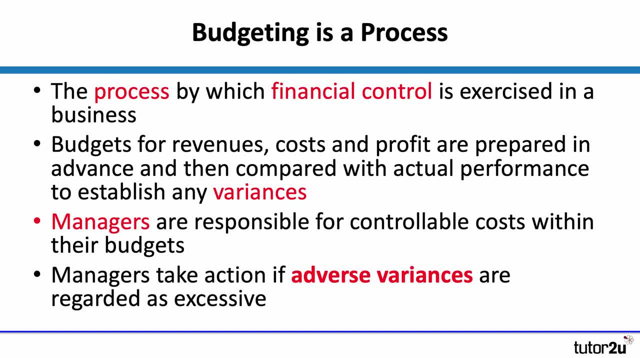 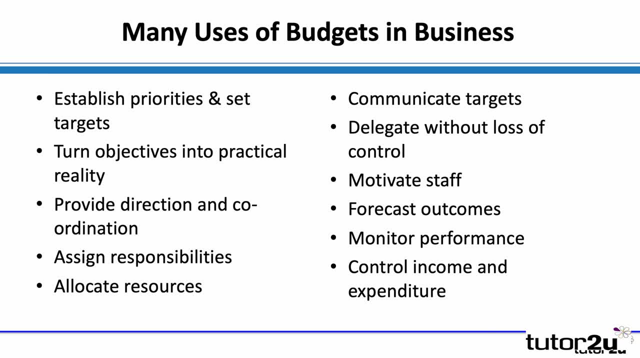 that managers in particular need to take account of and investigate as they arise. Now, budgeting is a very widely used process in businesses, And the reason for this is that budgeting has lots of different uses. You might want to pause the screen just for a second or two. just to list. 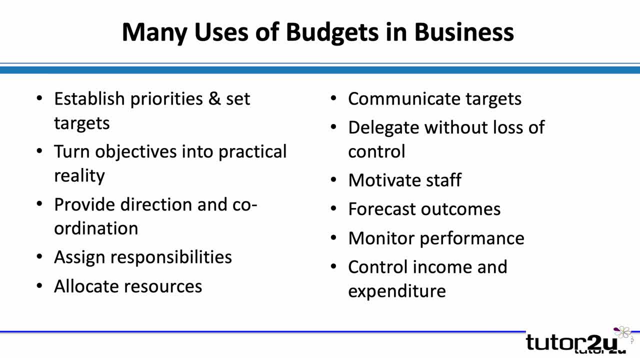 down one or two of them onto your notes, Picking out, I think, some of the most important parts of budgeting. I'd highlight this need for direction and coordination. Budgeting is a way of actually establishing the priorities of a business, allocating resources and then monitoring. 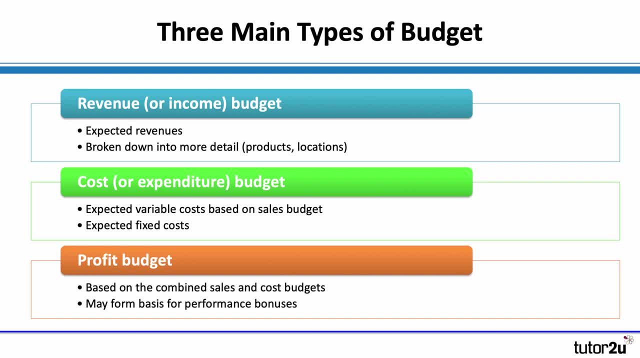 performance. There are three main types of budget. We've mentioned them already: The revenue, sometimes otherwise known as the income budget, which is all about the sales or the expected revenues, And often this will be broken down into much more detail, perhaps a budget by location, a budget by business unit or even 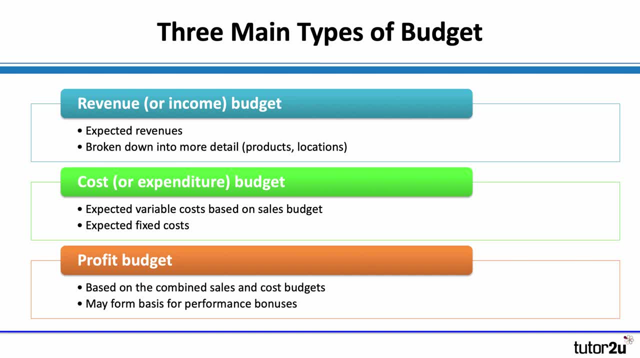 a budget by product. What you then do is you work out your cost budget, And this should be based on the sales budget, particularly applying variable costs to expected unit sales, But also this is where we include our fixed costs, the expected fixed costs, the budgeted fixed costs And, lastly, 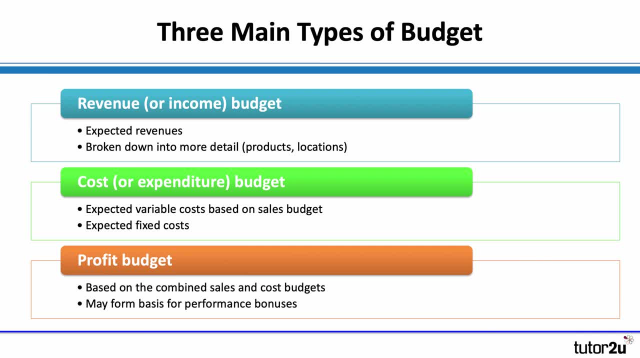 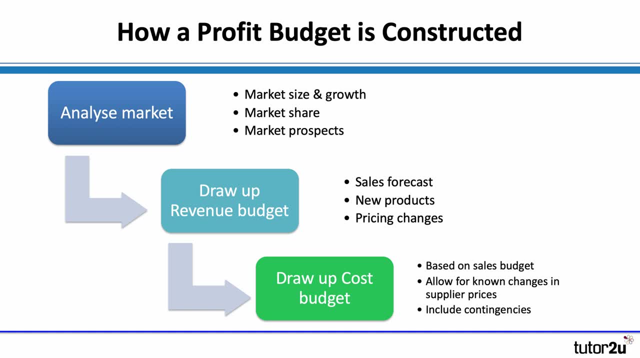 having done the revenue and cost budget, we can then work out the cost budget And then we can work out the profit budget. There's a process of putting a budget together and it's on the screen there. So, again, you may want to pause the video just to note down some key features of the process. 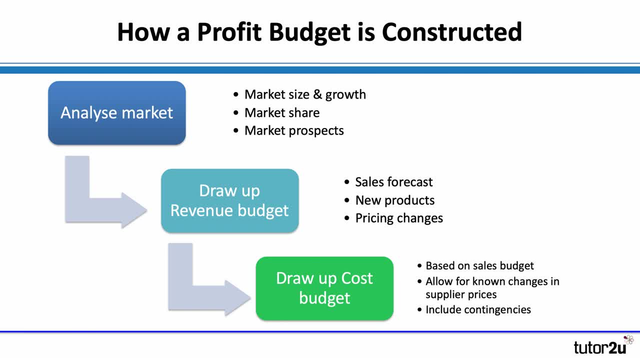 I would highlight the importance of starting with a market-based budget. There's no point just drawing up a revenue budget based on last year. You need to consider what's changed. How large is the market? How fast has it grown Or has it shrunk? 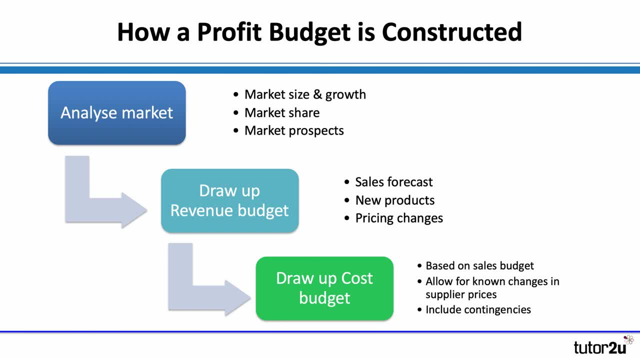 What's our market share? What are competitors doing? All of these are factors that you'd need to consider as you then draw up your revenue budget. A sales forecast or sales budget that's based on the latest information is likely to be much more accurate and useful than one that's. 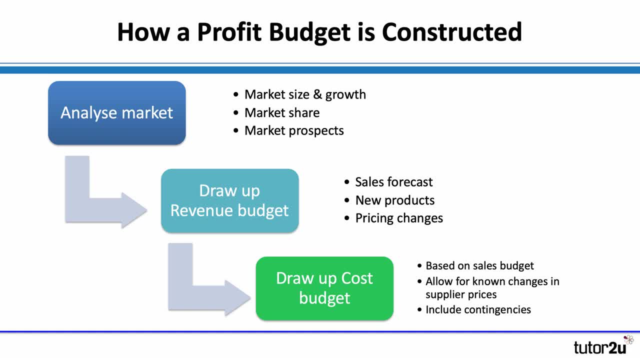 based on outdated assumptions. And similarly, when we're drawing up the cost budget, we need to make sure that we allow for some contingencies, some potential unexpected costs, as well as factors that are within our control, that we know about, For example, changes in the prices charged to us. 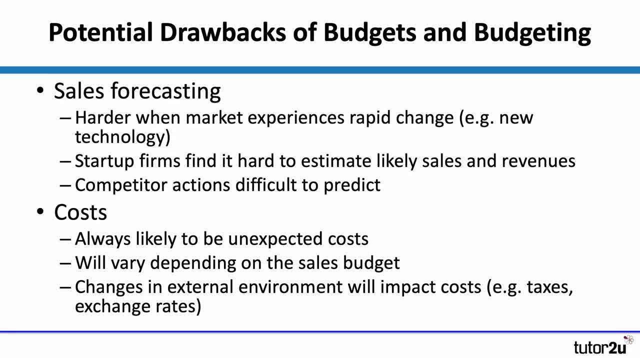 by suppliers. Well, budgets, budgeting, we've mentioned. it's a process And with all business processes, whilst they have their advantages, there are some potential drawbacks and some weaknesses, some limitations. Let's just look at the drawbacks first. Obviously, sales forecasting. 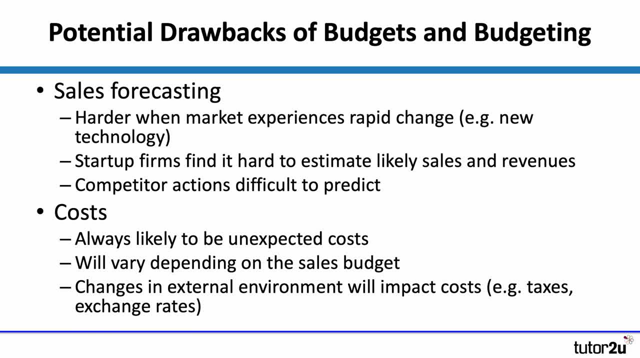 is at the heart of a budget And where markets change rapidly, for example through new tech or the actions of competitors, then it makes sales a lot harder to forecast. Where demand is uncertain, again that makes the sales revenue budget particularly difficult to put together. 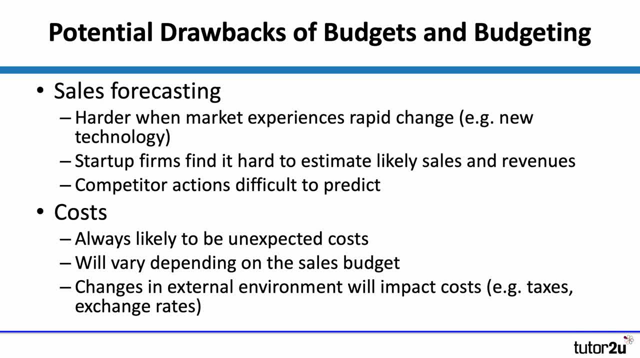 So I think with all budgets, you have to have an air of realism when putting them together. Similarly with costs. as we know, when we put our cost budget together, something is always going to happen that we didn't anticipate, And that could be good or bad news, For example. 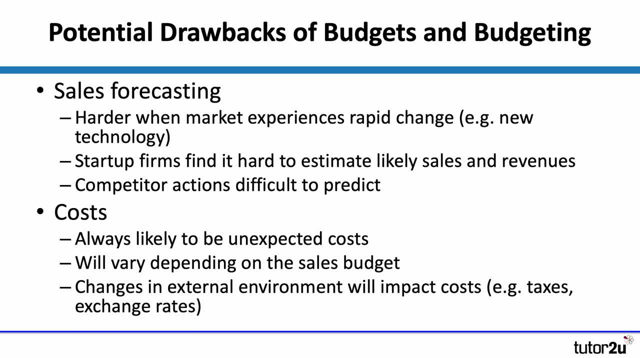 good costs might be a new product that you launched that you weren't expecting to launch in the original budget, And similarly, we need to be scanning the external environment to look out for changes which might affect our costs. Exchange rate changes is a great example of that, So any 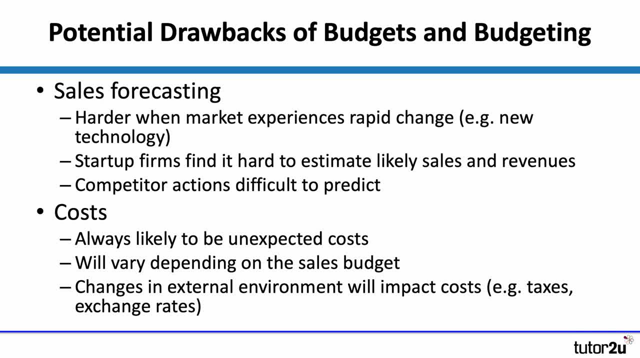 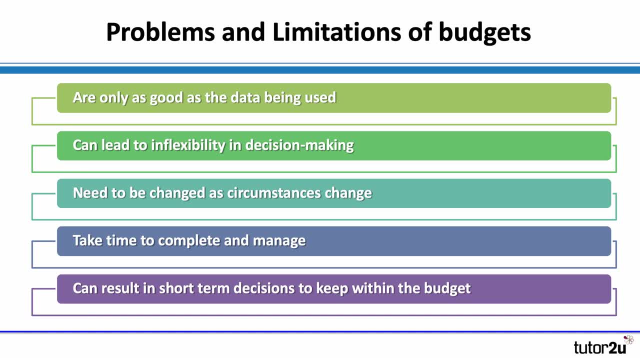 budget will assume a certain level of exchange rates, But of course, in reality, exchange rates will change during the course of the year And therefore it's just worth also noting down some of the limitations of budgeting. That's not to say that these